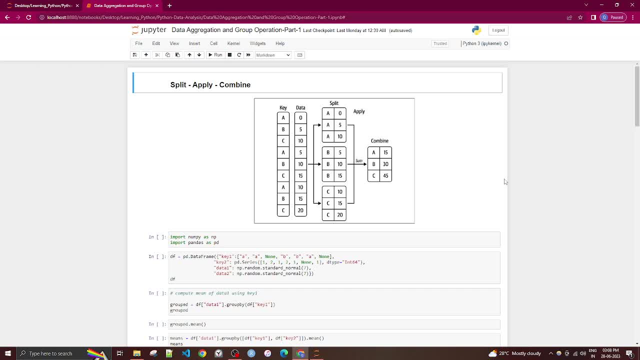 can write our own functions. So in this cup of video I would like to discuss on the data aggregation and the group operation and related function around those. So before I start, I want to also discuss one thing about this: split, apply, combine methodology, So what this means actually. 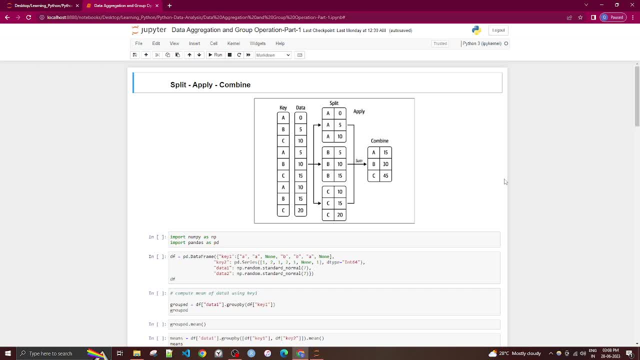 is when you do any group operation, right, any data aggregation, how the internal operation take place is where your data is there, right? It first let's get into grouped means it gets split, and then the operation. let's say you want to do the. 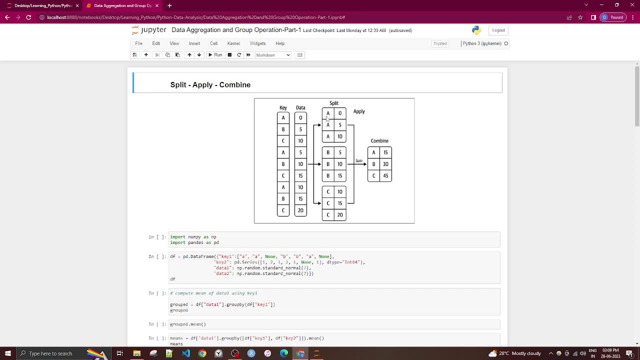 summation. So this is the data right And it is against. we are grouping based on the key. So we have ABC, ABC, three groups and now we want to sum it, So A will be summed into 15, right. And 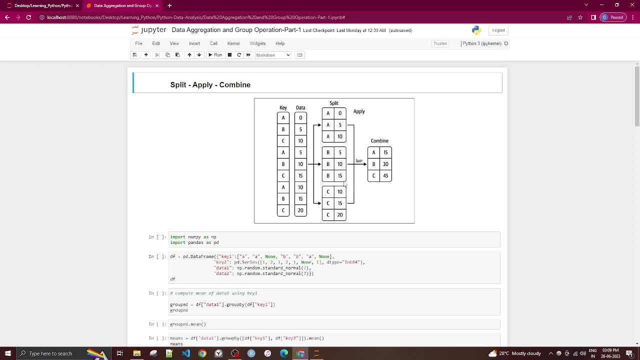 B will be summed into this 30, and C will be summed into 45. And then the last part is a combined, So all the group will be combined together to form one data. So this is a data frame or the series kind of a structure output in in in Python, right? So let's? 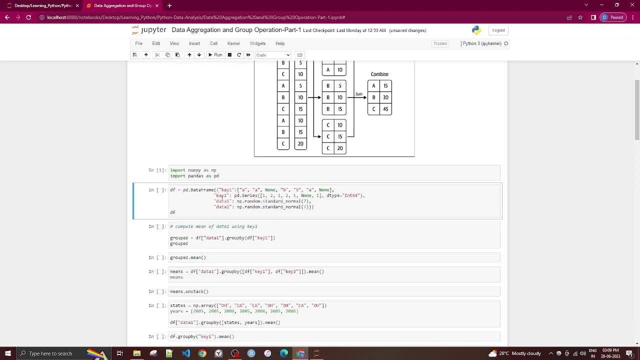 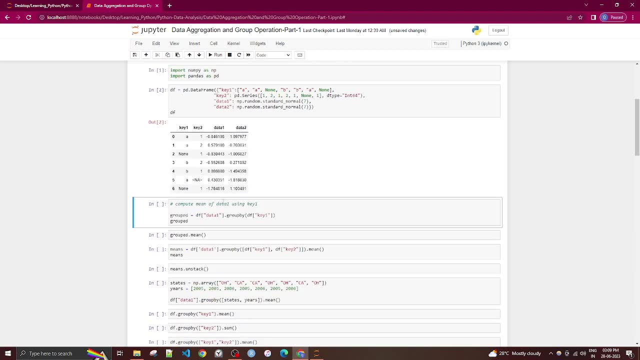 first start load our libraries and let's create one data frame. So in this we have key one, key two, data one and data two. So this is a data frame, right, And let's compute the mean out of it. So before we do that, let's group it. 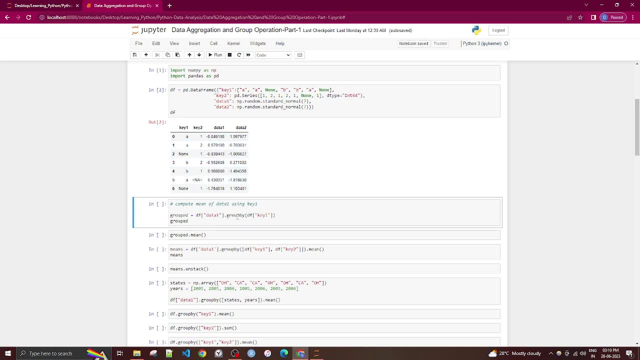 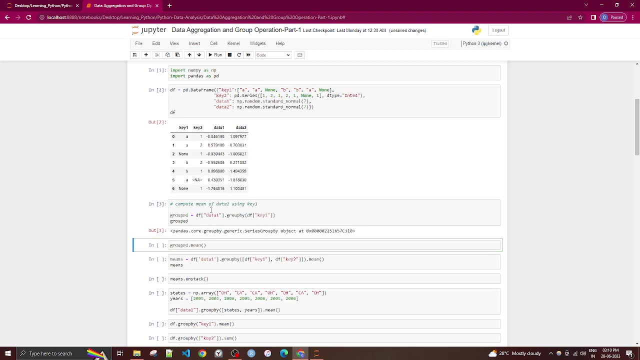 So what we are doing, we are data, we are taking one and grouping is based on the key one. so it will be a B group, right, And I'm putting that into the variable called group. So, as you can see it, we are supposed to see the 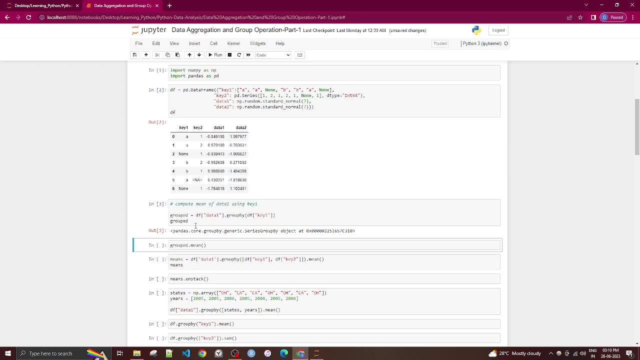 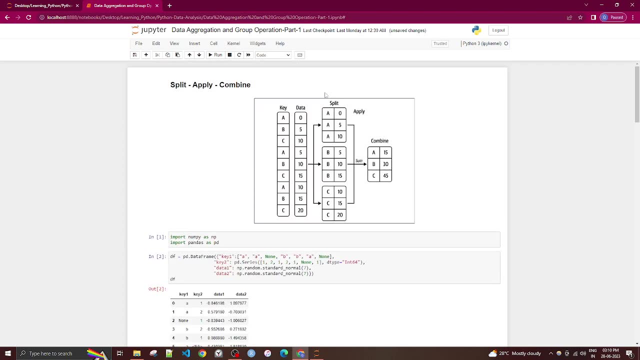 result. but it did not give us the result, what we weren't expecting, because it group means we are currently in this stage, in this state, and you can do more operation on on here. right, we eat already grouped and we will be doing mean of the group. So, as you can see in this A and B, 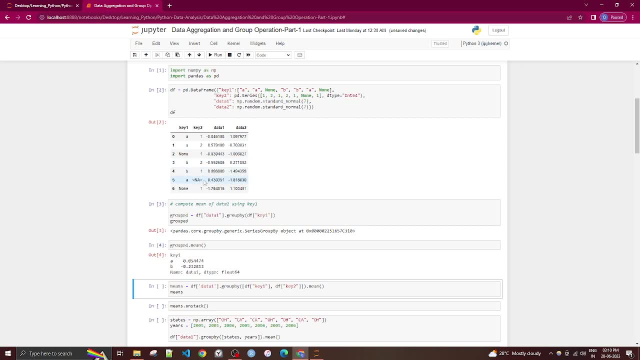 are the two groups and what it did. it provided the mean first. it group this and provide the mean of data one column. you can directly it. what is what we are doing? we are grouping data one again, group by key one and key two. so now a1 will be one group, a2 will be second group and we 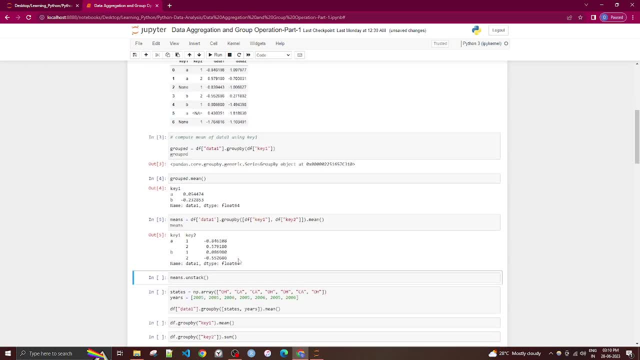 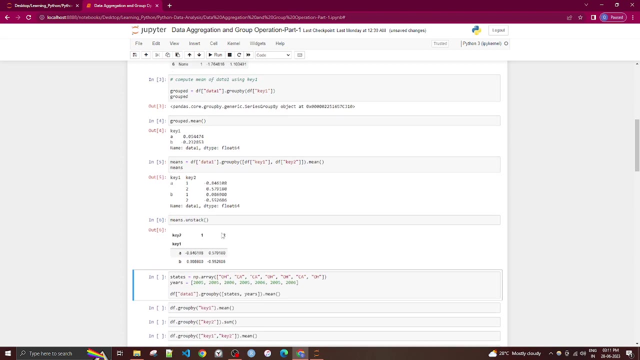 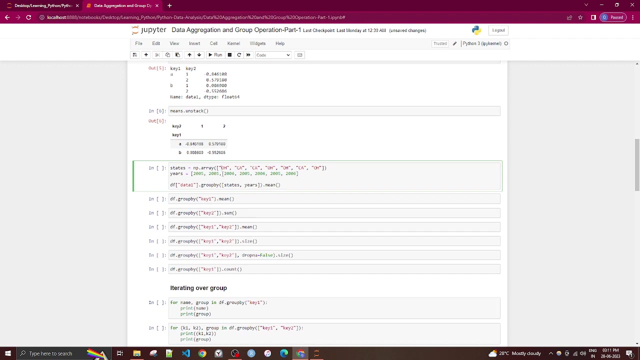 are doing the mean, so we are directly getting the result. this mean we can do the unstack right. we can convert. When the unstack happens, the inert key will convert in the columns. so let's move to next part of the it. we have this states and the years. 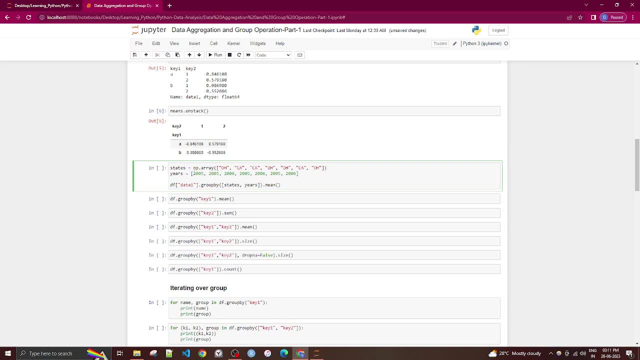 what we are going to do. we are going to do a grouping based on the state and years, so how it will happen. again, this is a part of the actual data, but you group outside the stack. So if you want to just take a look, that tools would taken out and it gets. consider this. 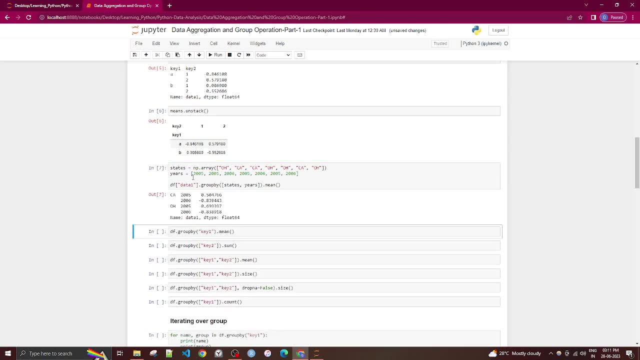 providing the additional list series and you can use that in grouping. so in this, CCAOH will be grouped based on, with respect to their years and the data. one will be grouped based on this particular state and the years indexes you can directly do the group by and create do the 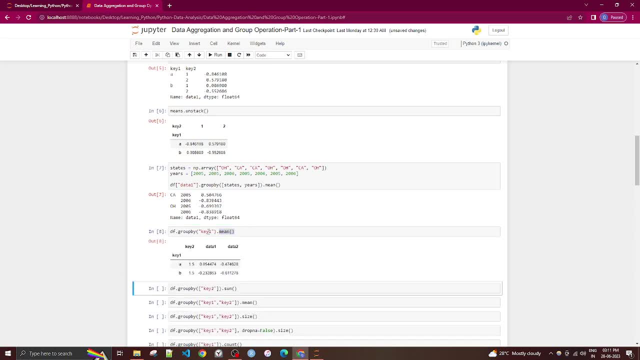 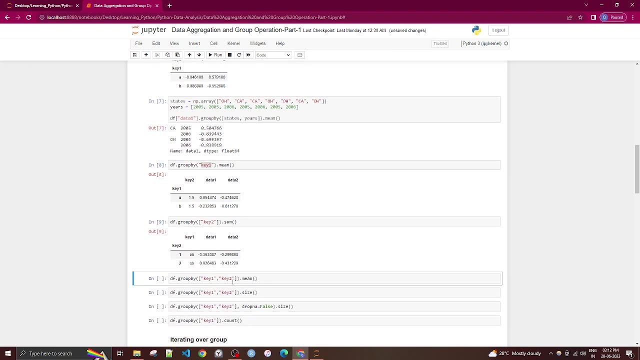 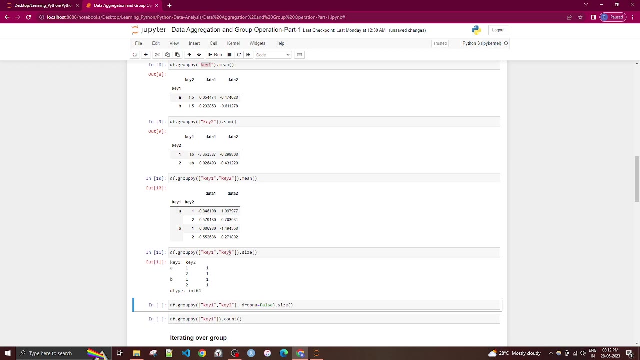 aggregation function like mean right. so what you do? group, group by key one, group by key one, and provide the mean of data one and data two, group by key two, provide the data one. you can again combine these two, key one and key two, and do the means right. you can also get the size and, as you can see, 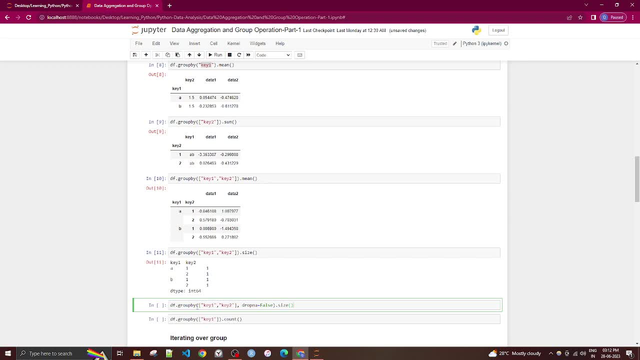 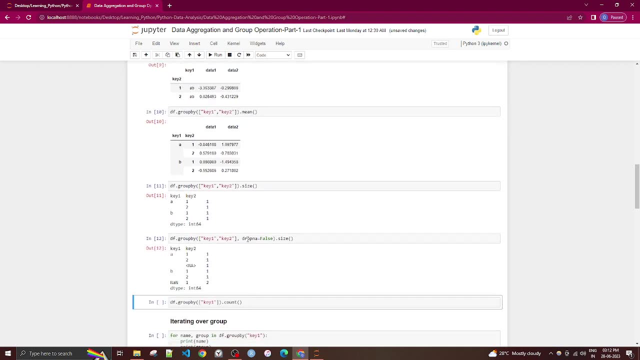 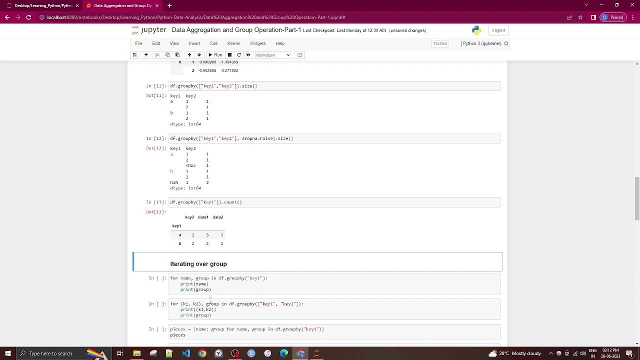 all this operation, the, the n is values are dropped, but if you want to keep the n is value, you can put additional values parameters, as you drop n equals to false and it will provide you the n is values too. again, you can do the counts operation also if you want to count the number of. 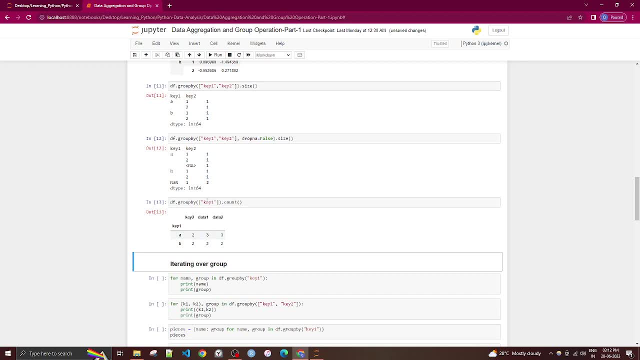 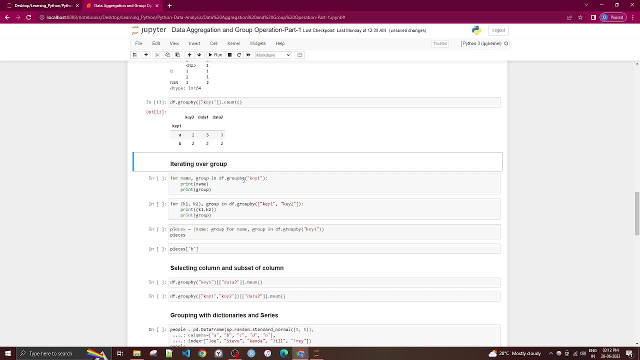 observation between data one and data two, based on the group by the key one. next, let's look at the iterating group power groups. so in the, in the key one, in the data frame, we have a. we are what we are doing. we are creating a group using the key one. 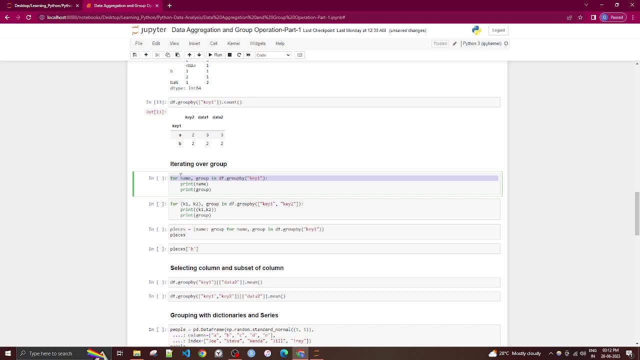 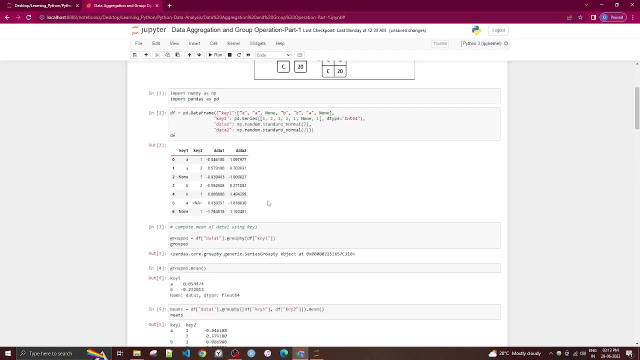 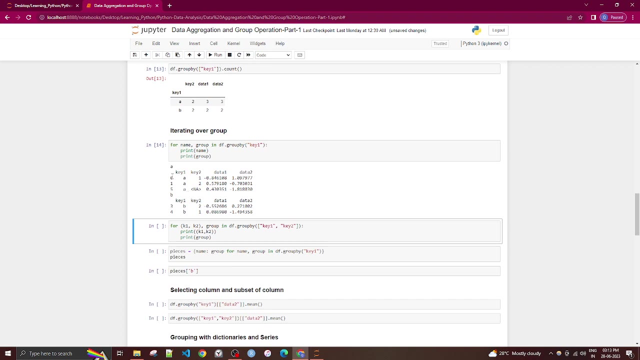 and we are iterating using the four loops, so name and the group, and first it will print the name and it will print the group. so we have two groups here, right, key one, if you, if i go up. so key one has two group a and b, right and a and b. and what it did? it just provided the first group, first the name. 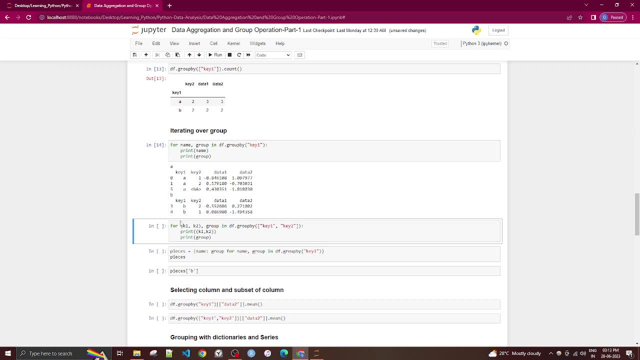 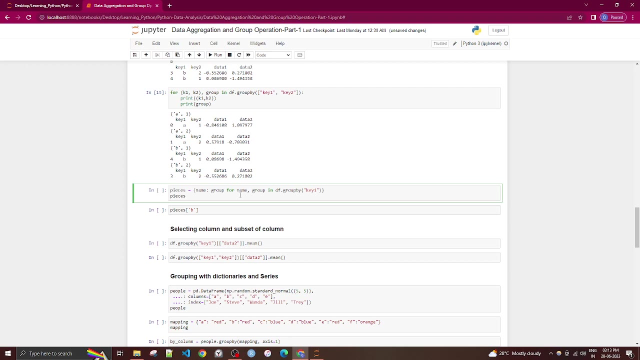 and then the actual group. all the data again. if you want to make a tuple, you can do that with group and first value, right group a1, a2, b1, b2 and this data. in this, what we are doing, we are again doing the for loop and creating a dictionary. so this is a 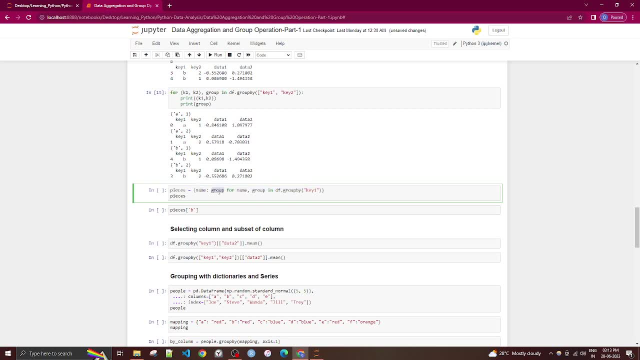 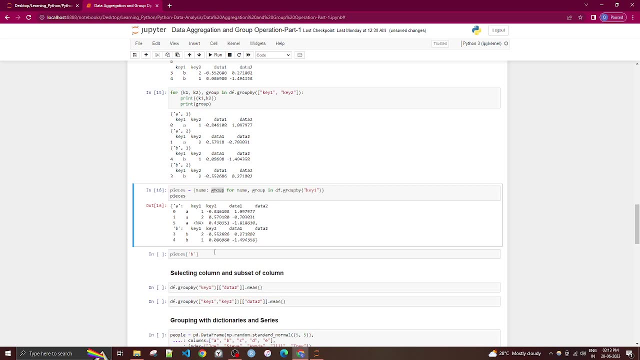 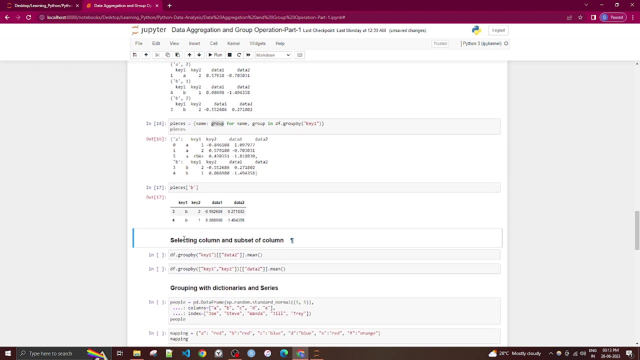 dictionary comprehension, where name and the group will be converted into the dictionary. this is a, first, it's key, and b and ski, and you can extract those you want to see on the b data. so this is all the b data. next, selecting the columns and subset of columns. so again, uh, this is the same thing which we did. 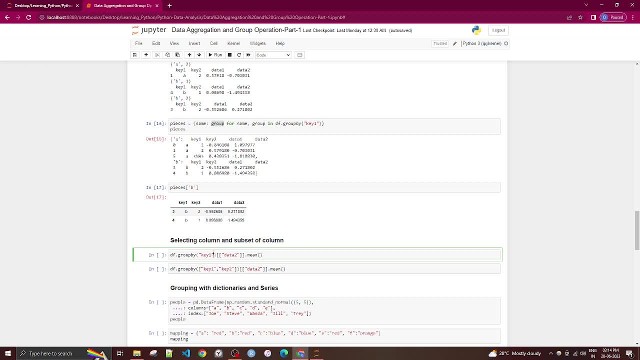 so if, if we have a group, we are doing the group one and we want to extract by group, after grouping the using the key key one, we can extract the key two and it's mean right. so again you have to put down your function. then only you can get the result, else we'll get the generic group by group. 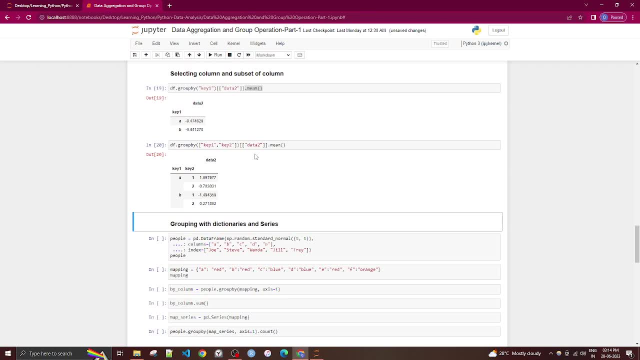 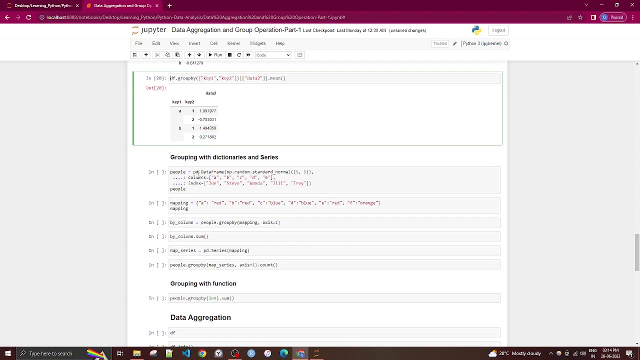 as the output. here we are expecting the data to based on the two keys right, key one and key two. as you can see, in this index we have key one and in the index we have key one can key two together. next is grouping with the dictionary and the series. again, let's create one, uh. 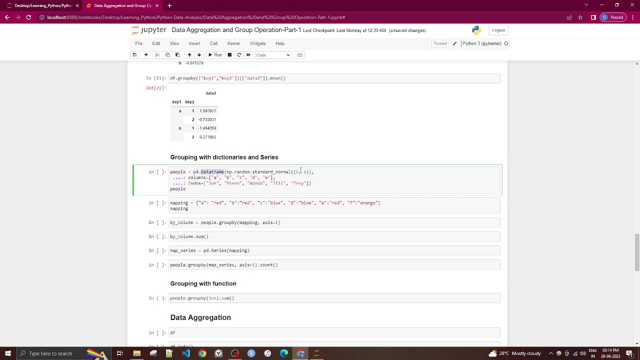 when data we have a data, one data frame. we have a data frame rate five into five matrix. the columns are e, b to c and the indexes will be jobs d1 to e b and the indexes will be just e 1 to e b. we have a data frame rate five into five matrix. the columns are a, b to c and the indexes will be 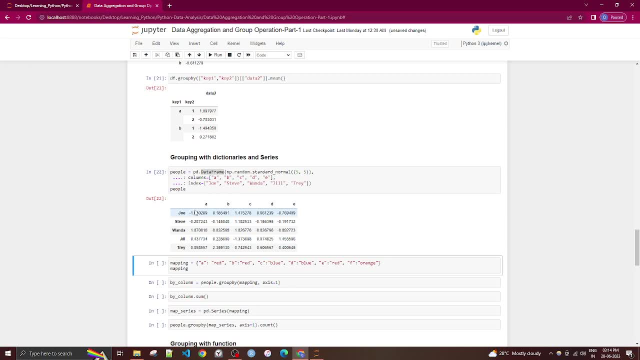 So this is what the data is and what we can do. we can create one mapping: a equals red, b equals to red, c equals to blue, and this is what we have, the mapping. so what you can do, we can group these people, people to group- by using this mapping, and we want to do mapping on axis, so a will be. 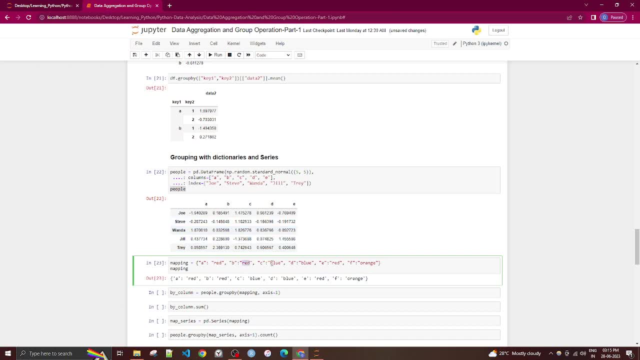 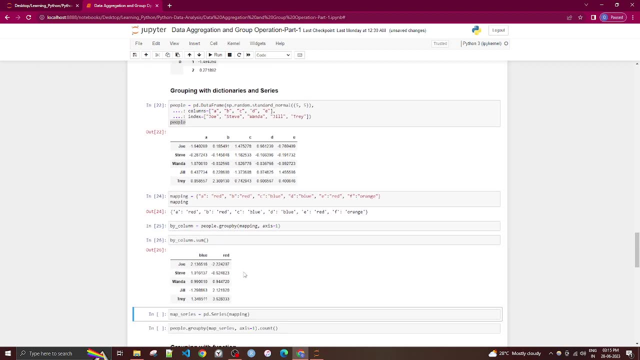 convert into red, be again red. C will be blue, blue, red, orange. so we have how many groups? three groups, right, and let's see. so we have okay. one thing I would like to highlight also, as you can see, why the third group is not there: because F. we have kept orange and there is no F, so that's why it. 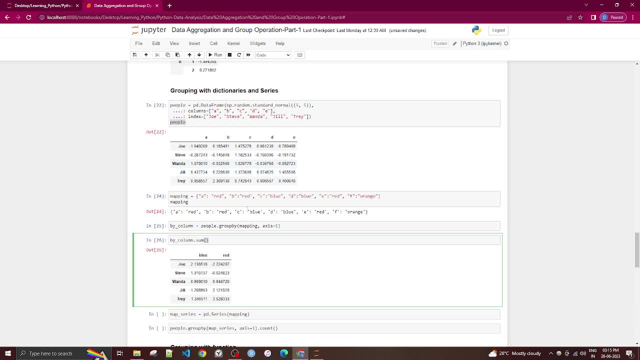 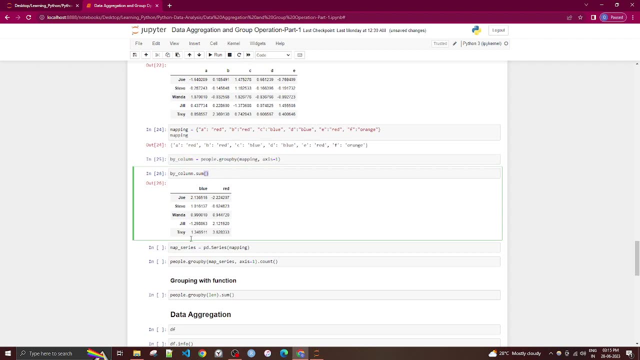 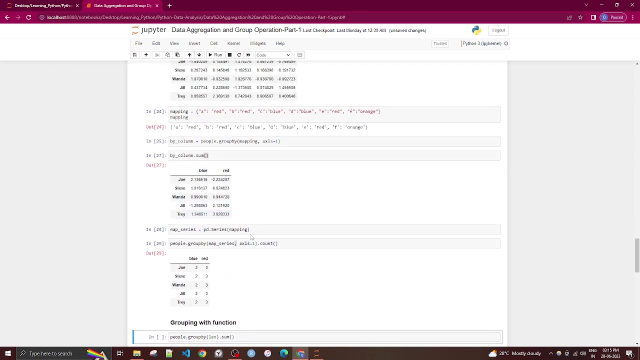 been discarded right. so now, if you remove the orange, then all the two group left is blue and red. you can do the. we can create the series and again use the series and count the number of the observation with the same result. so the idea here is: you can in the group by mapping. 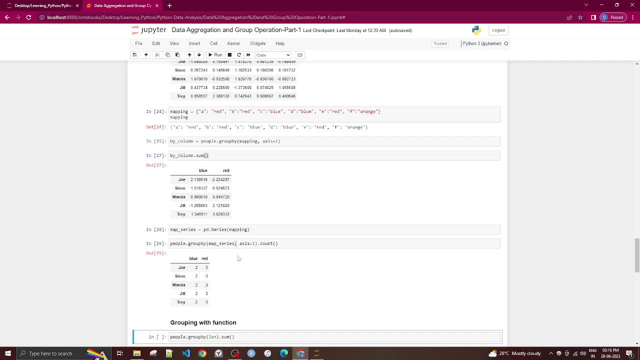 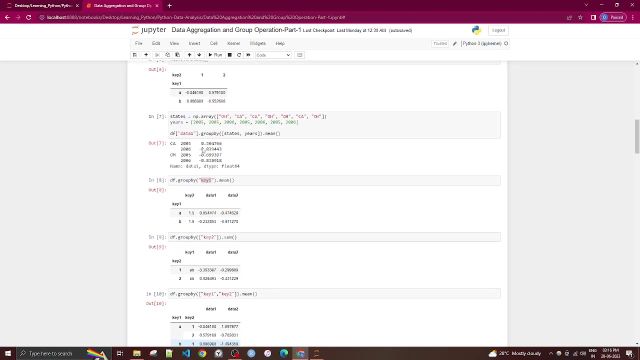 you can use any additional outer mappings, you don't have to use the existing one. or you can use the outer and, like in this case, we did the mapping right. we created one map in and also we above we did with the states and the names, right this one. so now let's 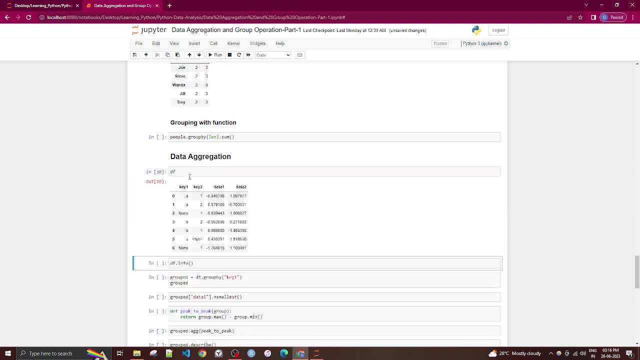 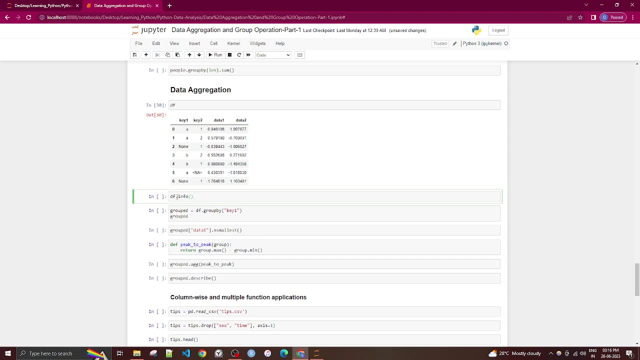 move into data aggregation. so we have this data frame right given key to data, one data and if you want to get the information of this data frame, there is a inbuilt function called data info, which is very efficient. it will give you all the title regarding the columns and let 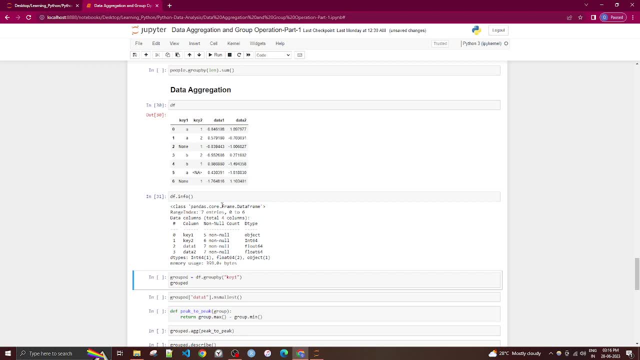 me run that first. so what we have here it's a class of the pandas code frame data frame. there are seven entries right: zero to six. zero to six. this is the index, then the columns. here there are four columns: zero, one, two, three. how many nonal values are there? so, as you can see in in this, we have two nonals. 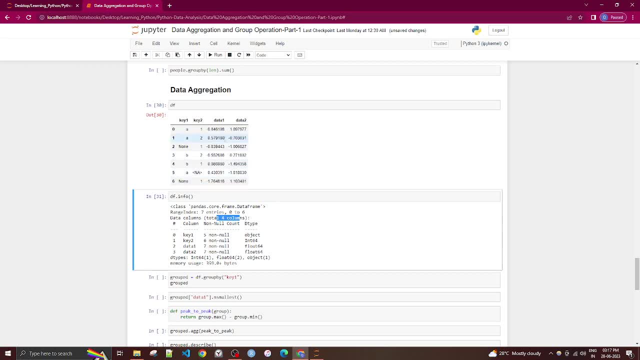 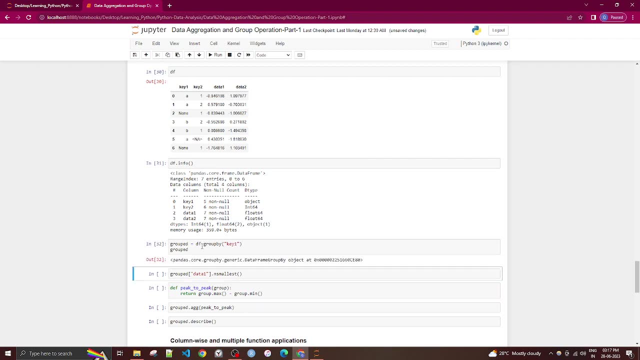 right, so five, you have one null, six and that there are no null, so it's a seven, seven values. so let's do the group by using the key. one right and it's a group, and on this group we can again use the uh, any other function mean some and 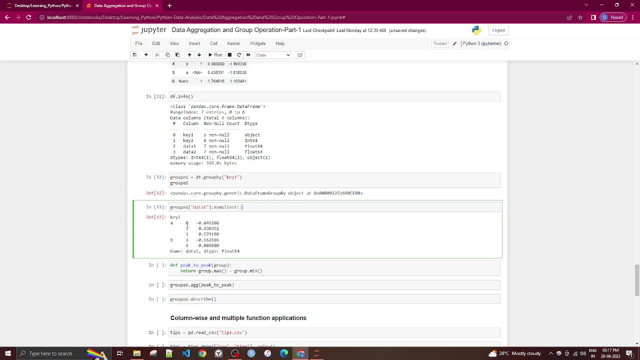 small, so it will give you the smallest function number in in that particular group. you can write your own function, like in this case. what I'm doing is, uh, peak. to peak means give the maximum and minimum and subtractor. so let's say the maximum value is hundred, minimum is ten. so the answer return. it will be going to return what- 90.. 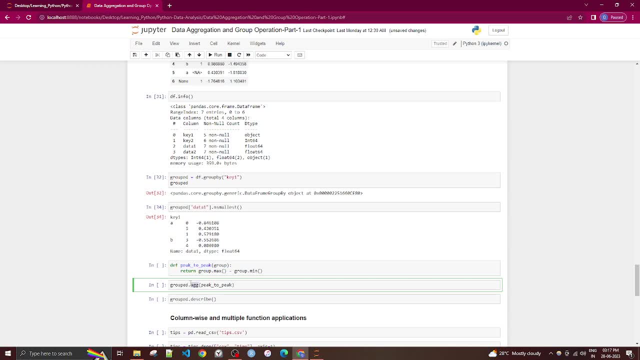 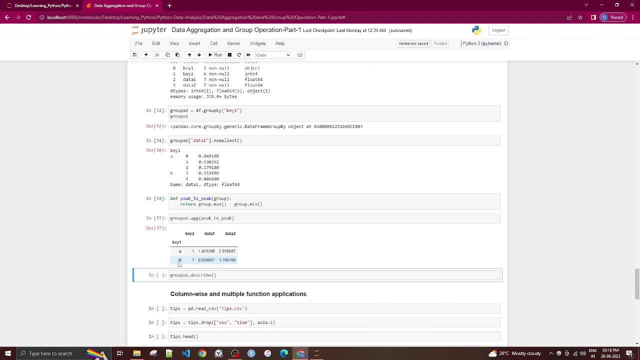 we are going to use agg, right, it's aggregated function and you can provide your inbuilt function or any uh diff user defined functionalize. in this case peak to peak, right, and it will give you. okay, let's run that and it will give you the result. so in this a and b, uh, key one, the difference between: 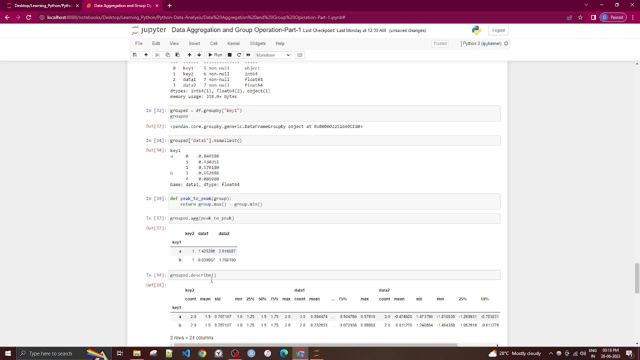 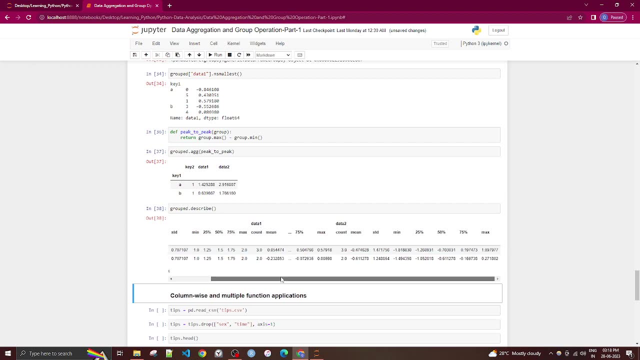 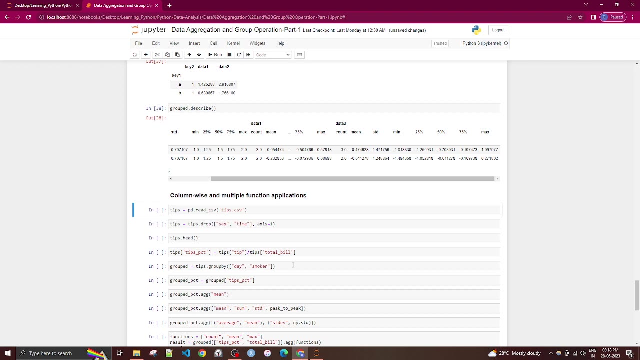 the maximum and the minimum is this, and again you can use describe. it will give you all sort of statistics. what is the count, means, standard, uh, quantize of the data one, and similarly for second group of the data two. let's do one example. so I have one data set: tipscsv. yeah, you can get it from the internet. 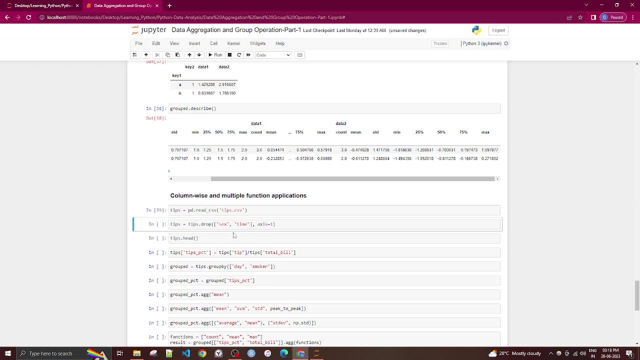 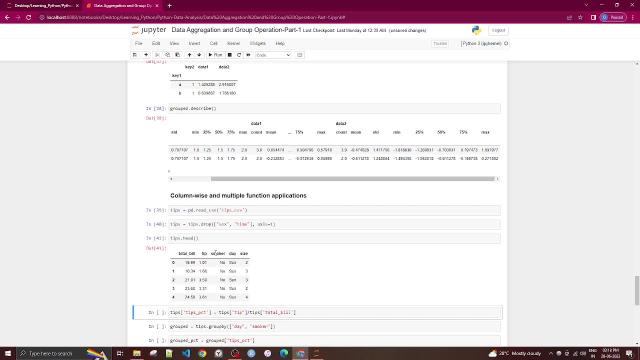 and let me load that and I will just drop this to sex and time columns and just let's see what the data set look like. so it has total bill tips- uh, whether the smoker day, and size, and let's add the third. now one more column. we are tip percentage. so T percent is what is the percentage of this tip based on the total? 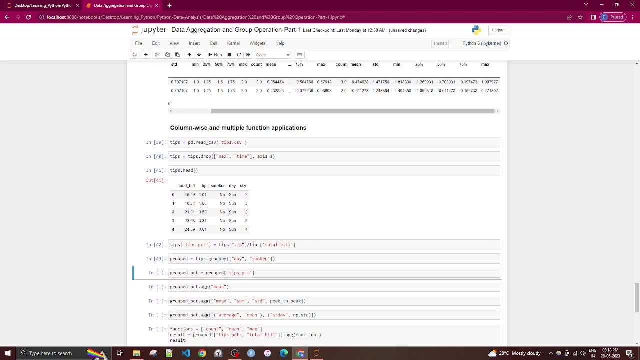 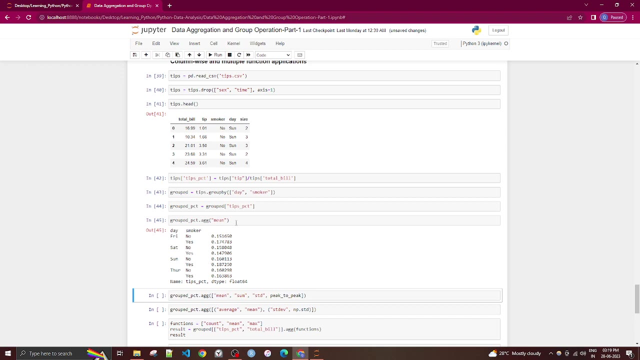 bill. now, I did what I did, I did group, I did group by based on the what D and smoker, right, and uh, let's run the aggregation here on the tips: BTC, right, this percentage. so we are, we grouped using date and day and smoker, and this is the mean of all these, all the of the two percentage. 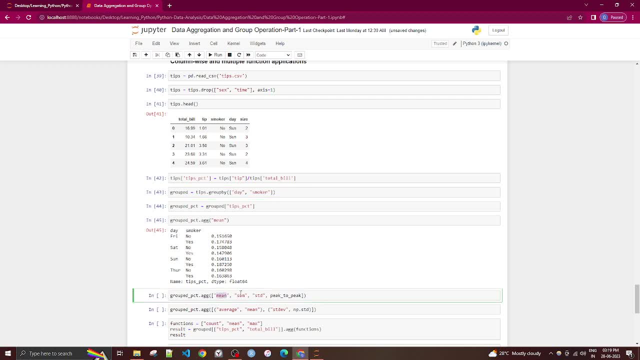 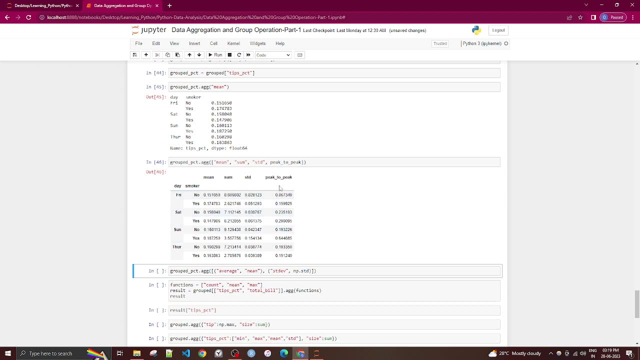 again, I told you you can use the AGG and provided the functions- multiple function- it will give you the result set on the day and smoker it means a mean, some standard deviation, peak to peak right, and if you want to change the names so you can provide average, so mean will be converted as the average and NPT is. 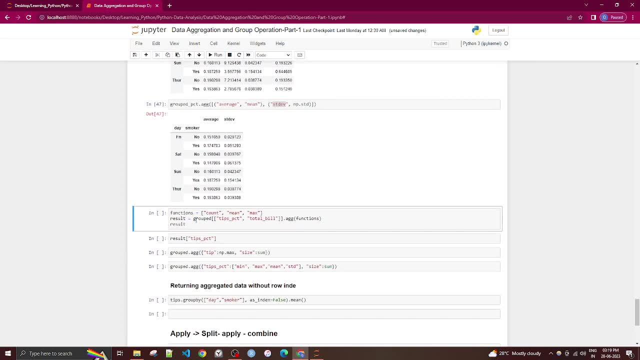 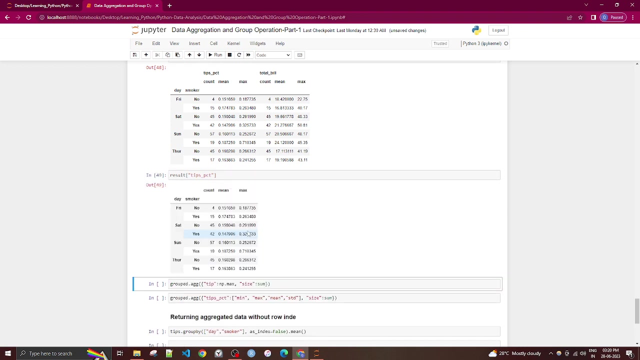 converted to standard deviation so you can create a list of all the functions, count, mean, max and provide that. so first group: I want to see only the grouped value of tips, percentage and total weight aggregated by this function and this is our results. look like right. and the next one: you can also use the. 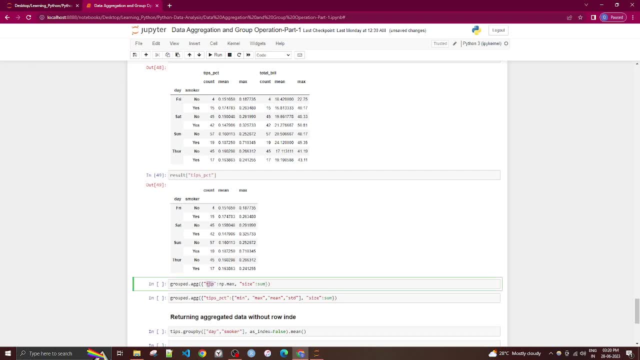 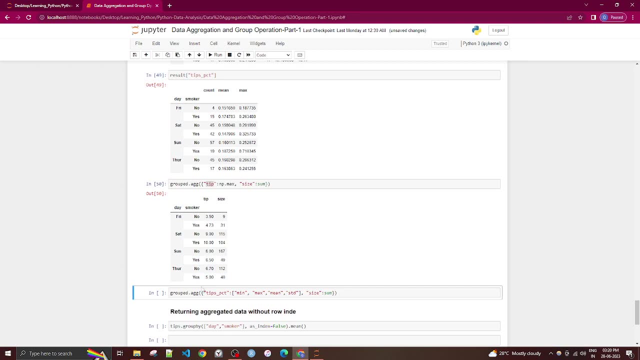 dictionary. so in the dictionary you can also use the dictionary. so in the dictionary you can also use the dictionary. so in the group if you want to see the maximum of tips and some you size you want to submit, right, you can provide again the multiple in the dictionary multiple. 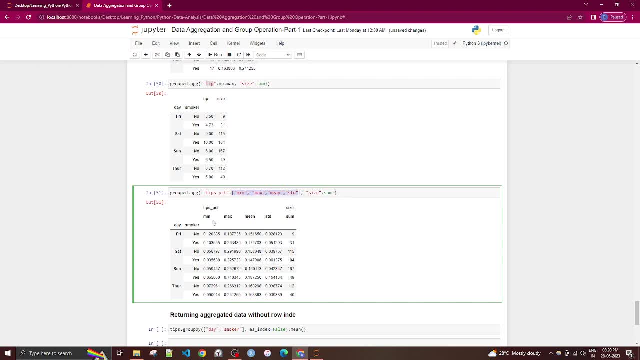 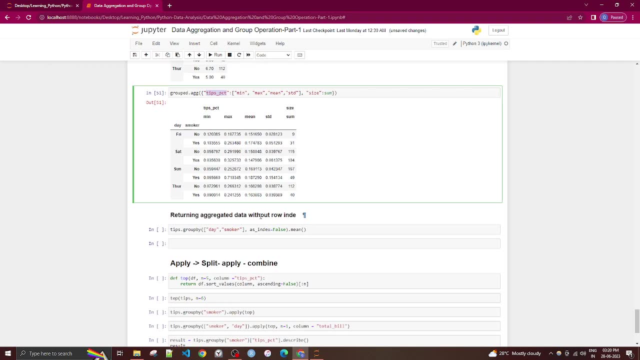 functions you want to apply to that group, and that's what is the other tips percentage: right, we want to see minimum, maximum, medium and standard deviation. next one is the returning data using without the row, so this is nothing but. next one is the returning data using without the row, so this is nothing but. 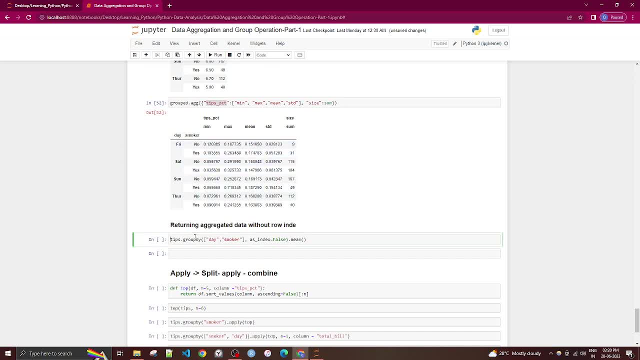 next one is the returning data using without the row, so this is nothing, but we have as index you can see that day and we have as index you can see that day and we have as index you can see that day and this mocos. right, so it just fill up the. 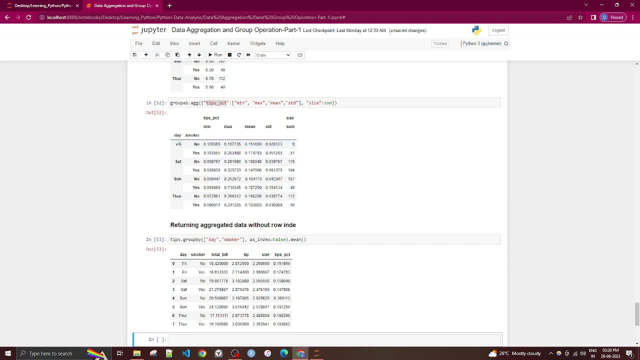 this, mocos right, so it just fill up the. this mocos right, so it just fill up the values on the index and move those index values on the index and move those index values on the index and move those index into the columns. okay, instead of what? 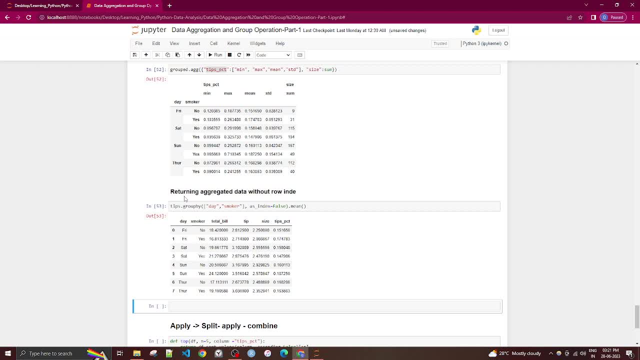 into the columns, okay, instead of what. into the columns, okay, instead of what exactly. it means you have whatever the exactly. it means you have whatever the exactly. it means you have whatever the group you have created, instead of seeing group you have created, instead of seeing group you have created, instead of seeing that into the index you can see as the. 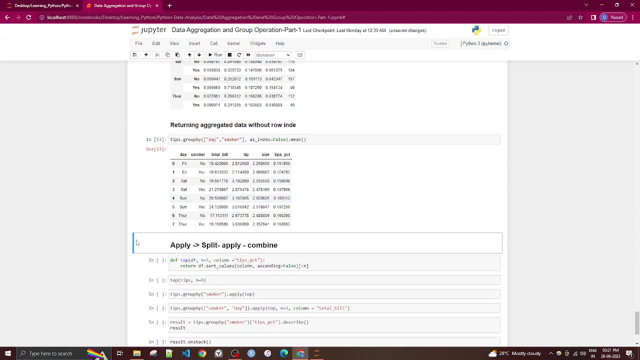 that into the index. you can see as the. that into the index you can see as the columns. okay, so let's also see the up columns. okay, so let's also see the up columns. okay, so let's also see the up. apply, split, apply and combine action. so 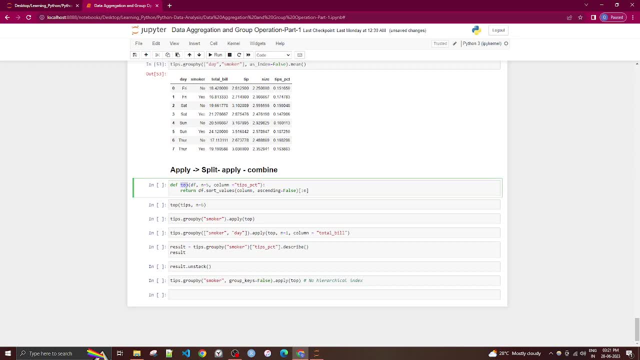 apply, split, apply and combine action. so apply, split, apply and combine action. so what I have created up, one user defined. what I have created up, one user defined. what I have created up, one user defined: function 2, where I'm taking input as the function 2, where I'm taking input as the. 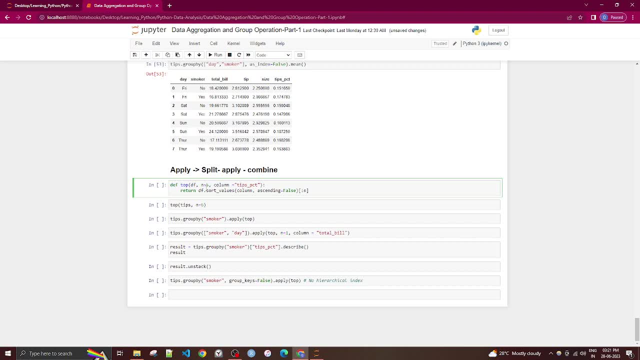 function 2, where I'm taking input as the data frame number of observation and the data frame number of observation and the data frame number of observation and the column and written. I'm returning these column and written. I'm returning these column and written. I'm returning these sorted values of that particular data. 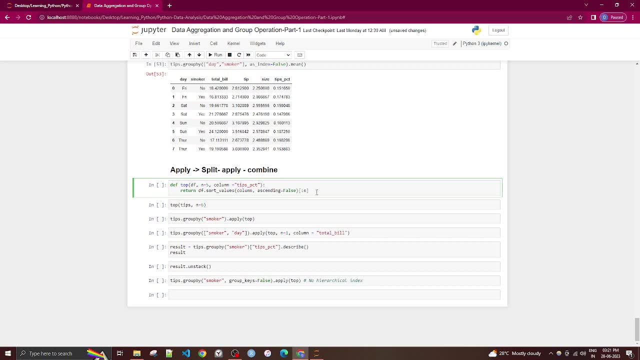 sorted values of that particular data. sorted values of that particular data. frame based on this column ascending is frame based on this column ascending is frame based on this column ascending is fall and it will show the numbers right fall and it will show the numbers right fall and it will show the numbers right. so let's- I'm applying tips- as the data. 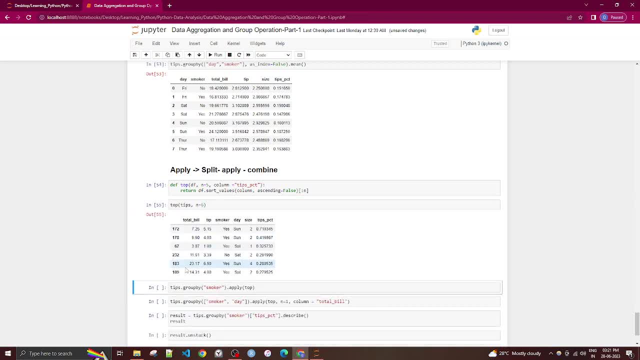 so let's, I'm applying tips as the data. so let's, I'm applying tips as the data. frame for six values, so T percentage. it frame for six values, so T percentage. it frame for six values, so T percentage. it shows from ascending to descending. so shows from ascending to descending. so 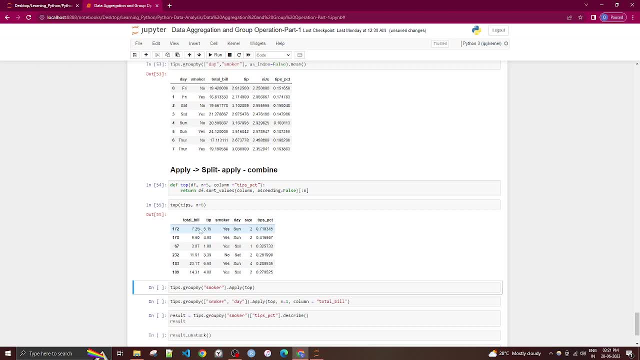 shows from ascending to descending. so this is the highest tips was given by. this is the highest tips was given by. this is the highest tips was given by: this. so the total peaceful 7.25 and the. this so the total peaceful 7.25 and the. 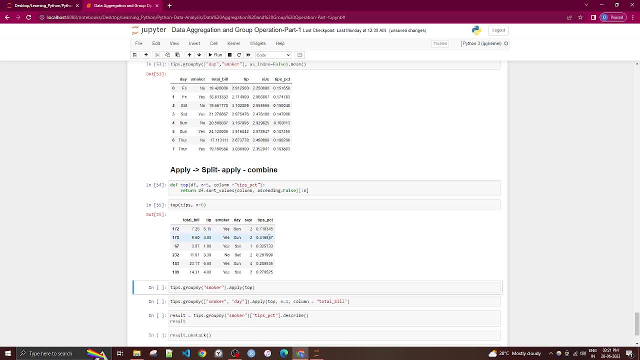 this. so the total peaceful 7.25. and the tip was giving five point one five. so tip was giving five point one five. so tip was giving five point one five. so that's the like, almost 70%, 71% of the. that's the like, almost 70%, 71% of the. 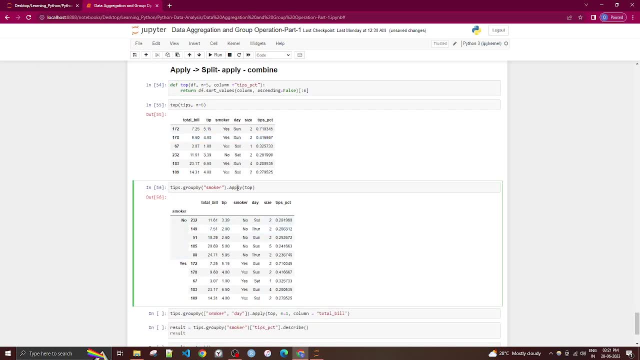 that's the like. almost 70%, 71% of the tip was given right. you can apply again. tip was given right. you can apply again. tip was given right. you can apply again. you can apply. apply is the inbuilt. you can apply. apply is the inbuilt. 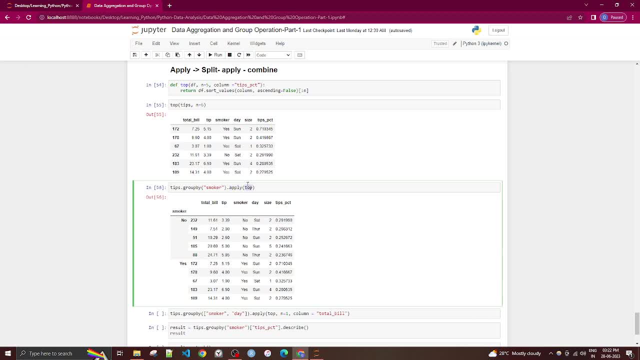 you can apply- apply is the inbuilt function and you can provide the top function and you can provide the top function and you can provide the top right this user defined function and right this user defined function and right this user defined function- and will give you all the results set based. 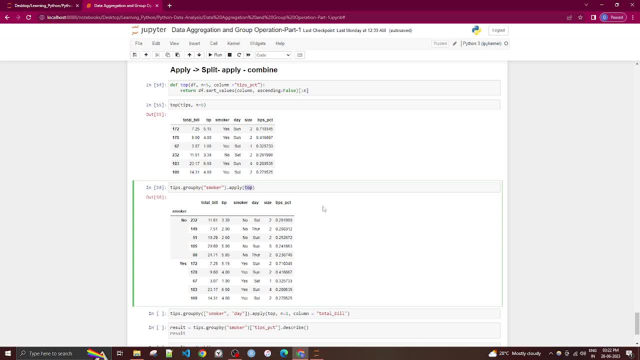 will give you all the results set based. will give you all the results set based on the smoker. a smoker is a group by: on the smoker. a smoker is a group by: on the smoker. a smoker is a group by and it on all the other existing column. 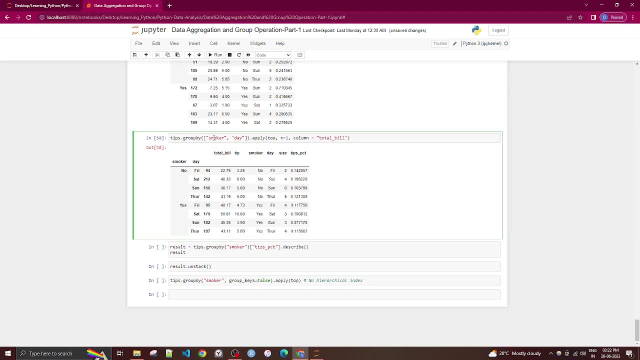 and it on all the other existing column and it on all the other existing column in the data frame. similarly, I am just in the data frame. similarly, I am just in the data frame. similarly, I am just using the smoker entities applied- apply. using the smoker entities: apply- apply. 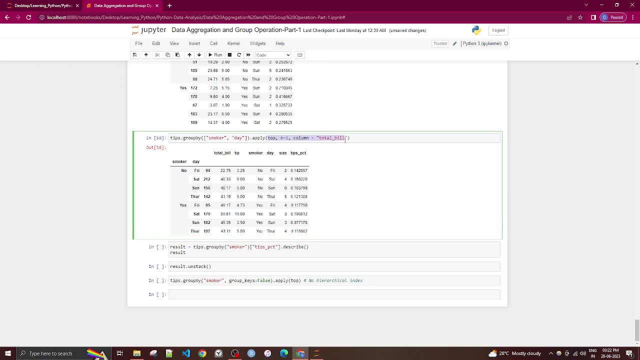 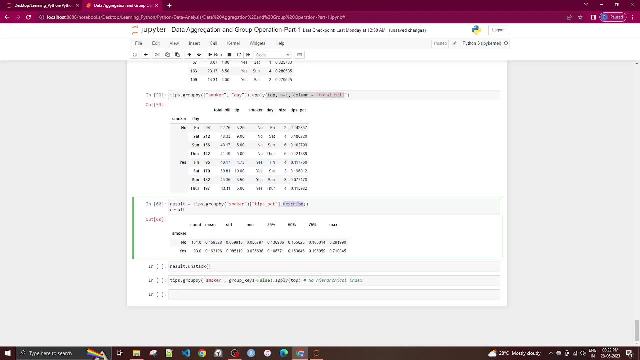 using the smoker entities apply: apply. and providing the other arguments in the. and providing the other arguments in the. and providing the other arguments in the tops describe: I've already discussed, so tops describe: I've already discussed, so tops describe: I've already discussed, so you can. you can first group it and tell. 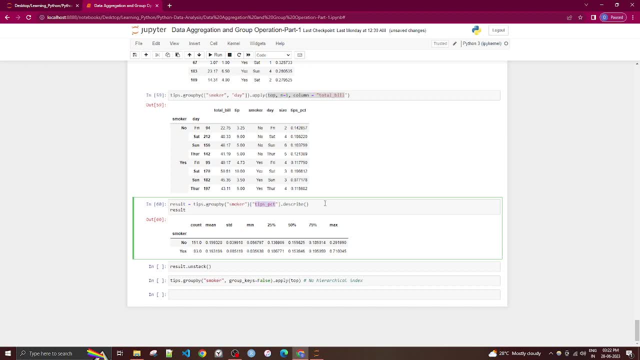 you can. you can first group it and tell you can. you can first group it and tell the right. then on which column you want the right. then on which column you want the right. then on which column you want to see the inbuilt statistics from the. to see the inbuilt statistics from the. 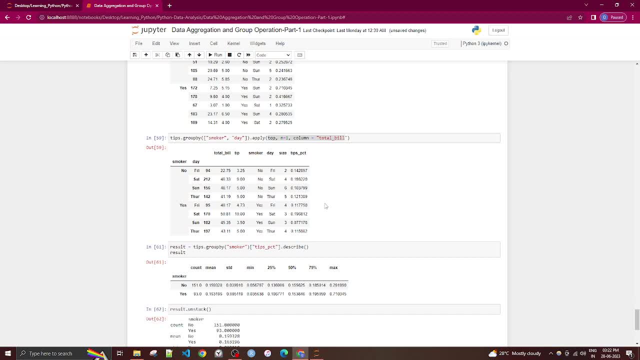 to see the inbuilt statistics from the described function. that's how you can described function. that's how you can described function. that's how you can and you can do the on stack of this and you can do the on stack of this and you can do the on stack of this right. converting your columns into rows. 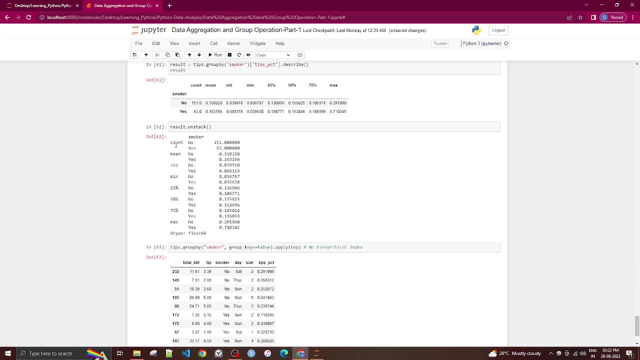 right converting your columns into rows. right converting your columns into rows. and. if you don't want to see the and. if you don't want to see the and if you don't want to see the hierarchical indexing, you can just apply. hierarchical indexing: you can just apply. 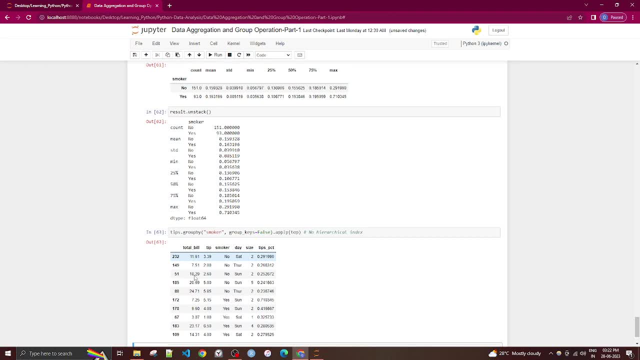 hierarchical indexing. you can just apply directly group fall group key equals to directly group fall group key equals to directly group fall group key equals to false, and it will remove the indexes and false. and it will remove the indexes and false. and it will remove the indexes and only show you the, the numbers, the index. 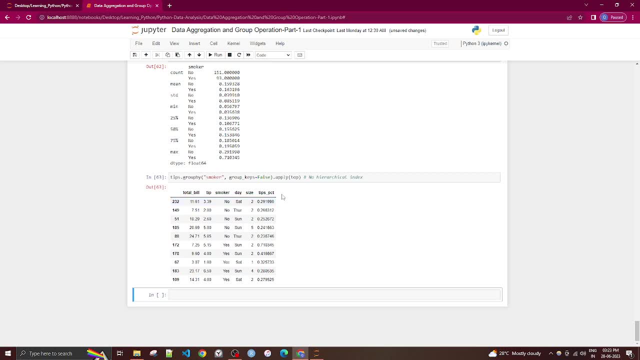 only show you the, the numbers, the index only show you the, the numbers, the index number, and with the other columns in the number and with the other columns in the number and with the other columns in the data set. so there are a lot of function, data set. so there are a lot of function. 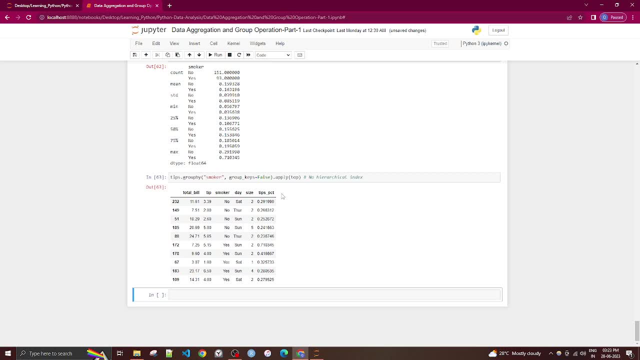 data set. so there are a lot of function. we covered in the data aggregation and we covered in the data aggregation and we covered in the data aggregation and the group operation. I have one more: the group operation. I have one more the group operation. I have one more video. I will showcase and continue our 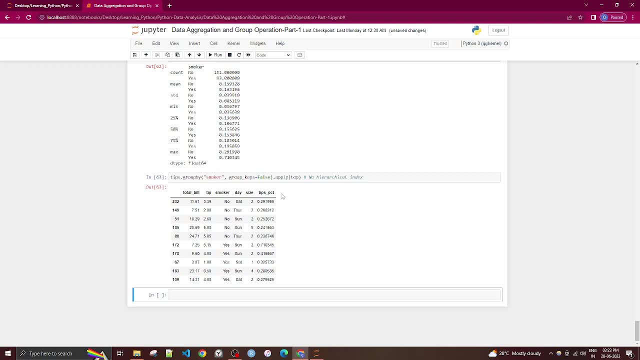 video. I will showcase and continue our video. I will showcase and continue our discussion on this group operations. discussion on this group operations. discussion on this group operations using the inbuilt and the user do it using the inbuilt and the user do it using the inbuilt and the user do it function. thank you,